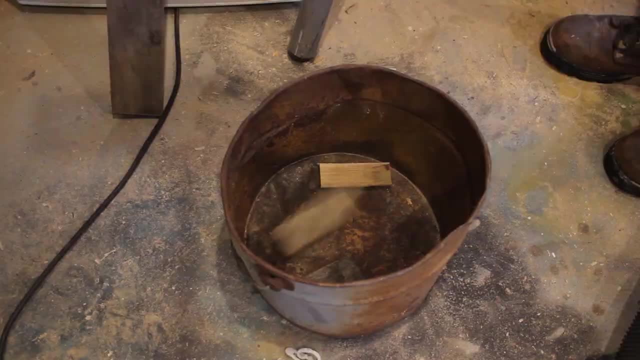 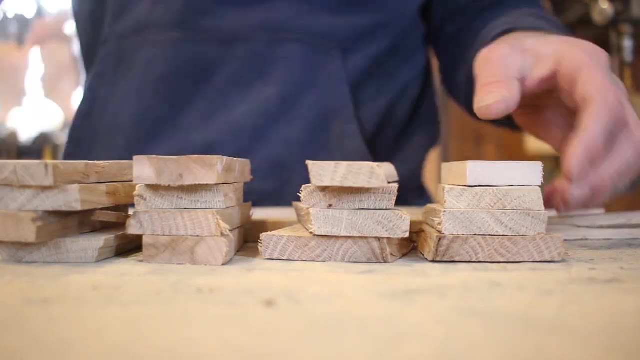 to start splitting them. Splitting these boards with an axe just gives the finished product a rustic or natural look, I guess. Once I had all my individual bottle openers cut and ready to go, I moved on to the drill press to drill out the spot where the bottle top will slide. 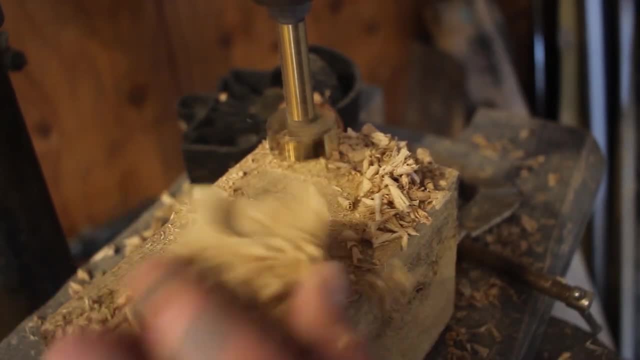 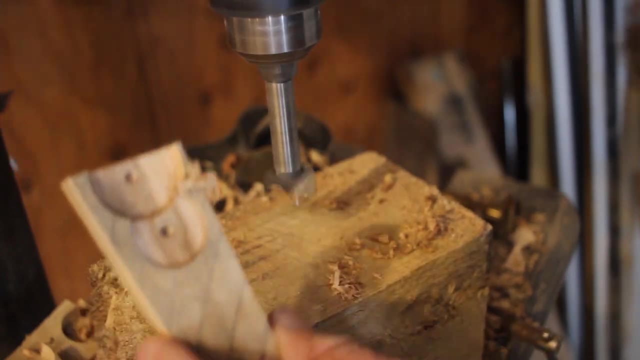 into the opener. I used a forstner bit for that and then moved on to drilling a smaller hole right behind that hole I had just drilled. You're going to want these two holes to slightly overlap, just like that. The depth and size of this hole is predetermined by a washer. I'm going 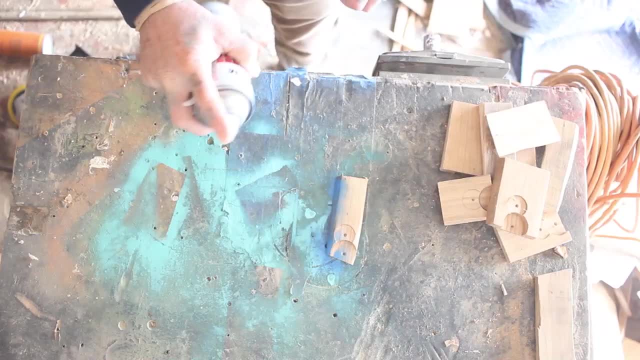 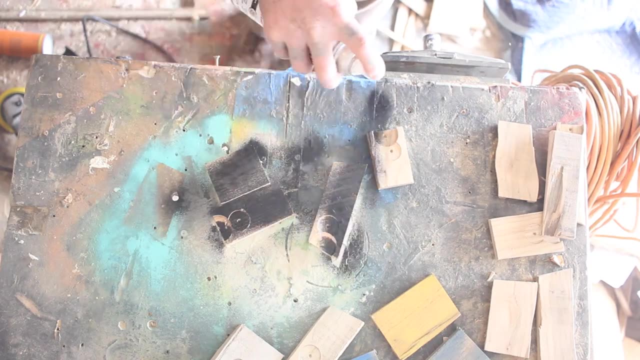 to be placing into that hole. After I was done drilling all these holes, I decided I would give some of these bottle openers a little bit of color with some spray paint. The idea here is to just give them a little bit of light paint and then go back and sand. 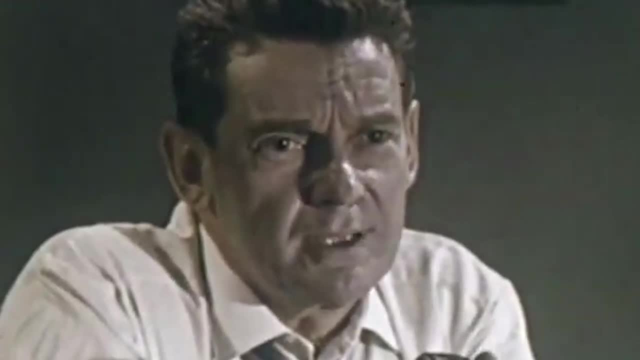 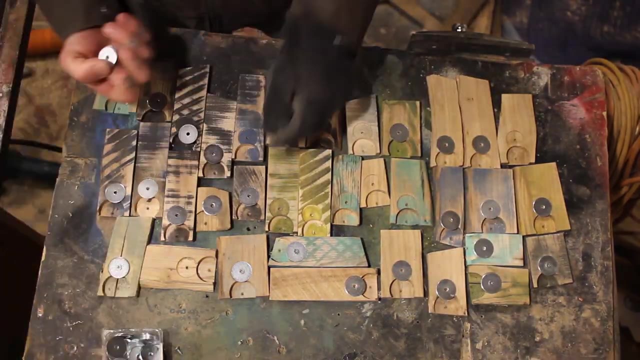 most of it off. Perhaps you're wondering why I'm telling you all this and I wonder myself. Now that I had them all sanded and ready to go, I laid them out and pre-drilled all my holes. I placed a washer in each one of these and then, using these small screws, I tightened. 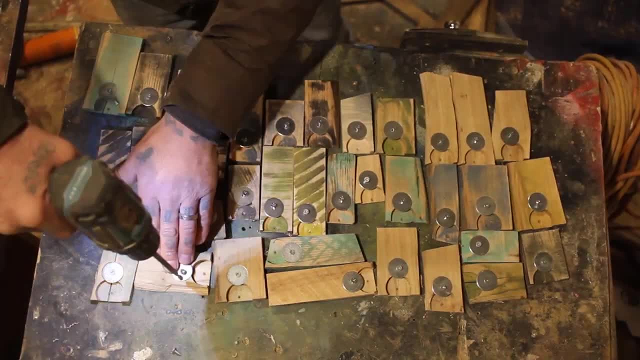 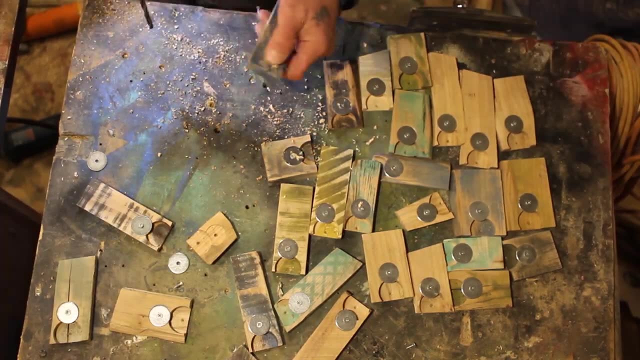 them down. I should have put a dot of super glue in each one of my screw holes before I tightened the washers down, so the washer would be less likely to pull out. but I forgot and I went back and did it all off camera. 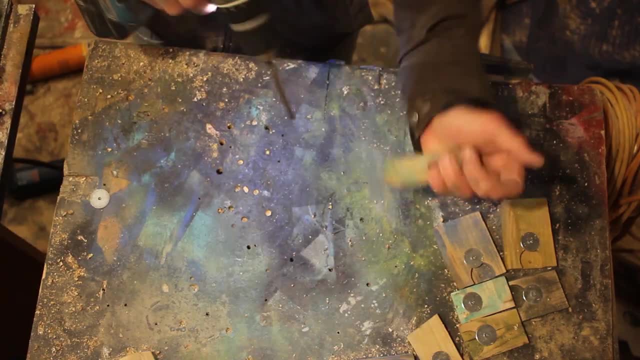 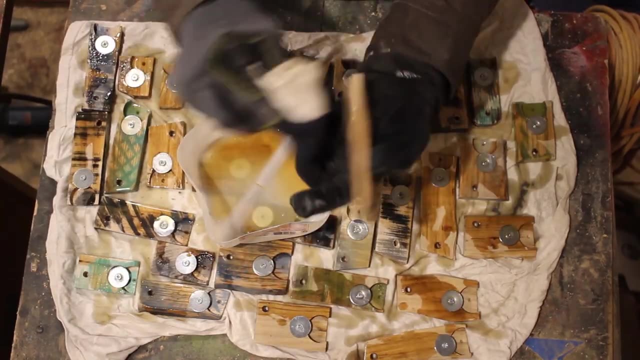 Don't skip this step or you'll have a lot of upset customers. This is also why you can't use pine. The pine wood is too soft and that screw will pull right out. I drilled a hole in the back of every single bottle opener and then sanded around the hole. 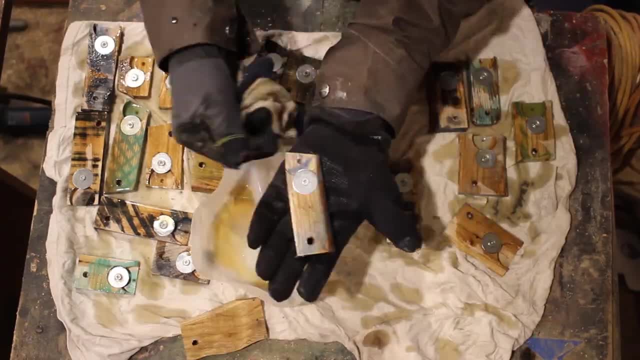 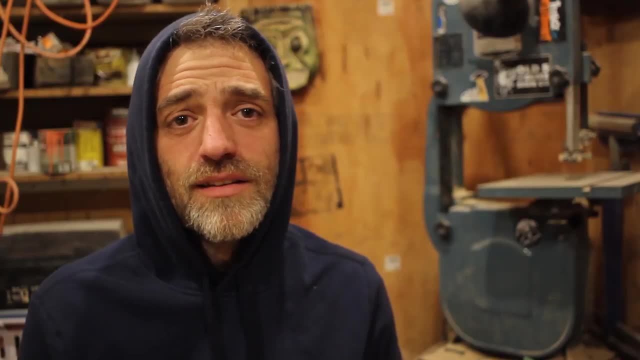 so I could put some paracord in there and have a way to hang the bottle openers up. I sell these bottle openers for $5 at a craft fair or $2 for $7, and they sell. This is an easy project that anybody can do and a fast way to make money from some garbage. 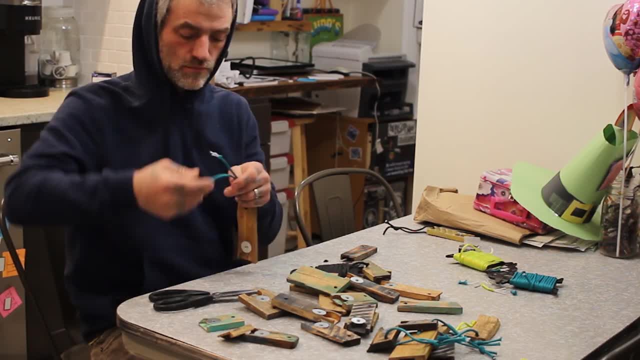 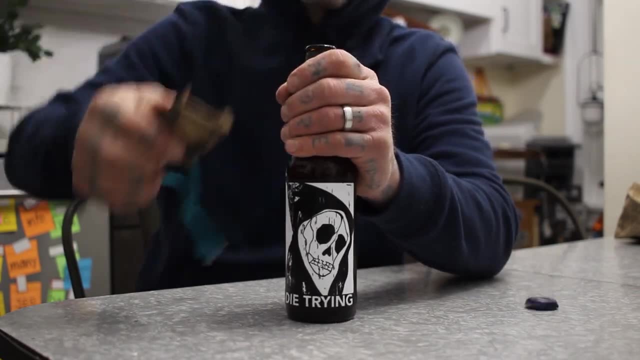 Once I had them all ready to go, it was time to bring them in and tie some paracord around each one of them. Now all that's left to do is test each and every one of these. Wish me luck. Thank you, guys. so much for watching, Like, subscribe, share all that fun stuff and I'll